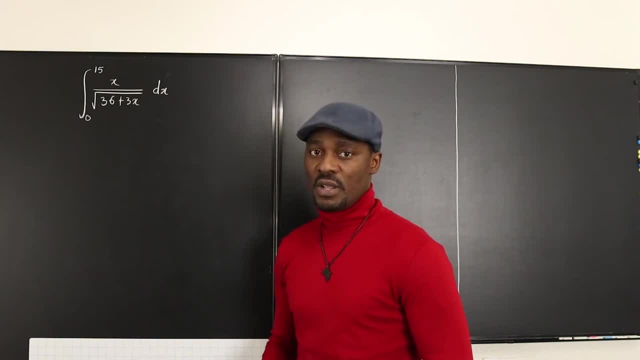 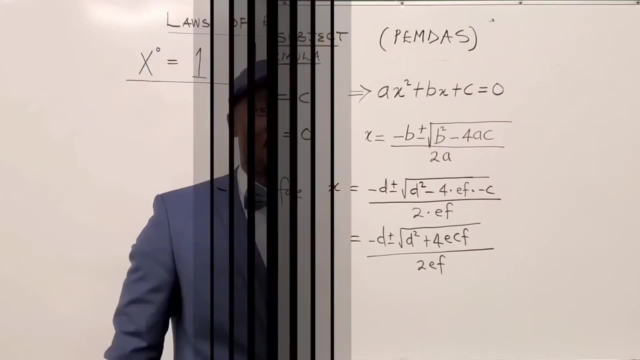 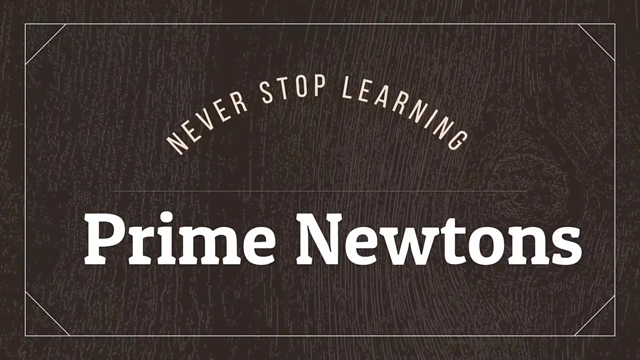 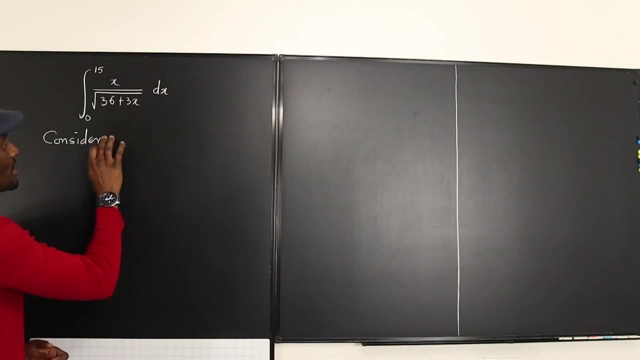 you might just start thinking of doing a? u substitution. So let's just go ahead and do this. So we're going to say to consider, because we don't want to keep taking this 0 and 15 together. okay, because that's going to be a lot of writing. You just want to rewrite this expression and say: consider the expression. 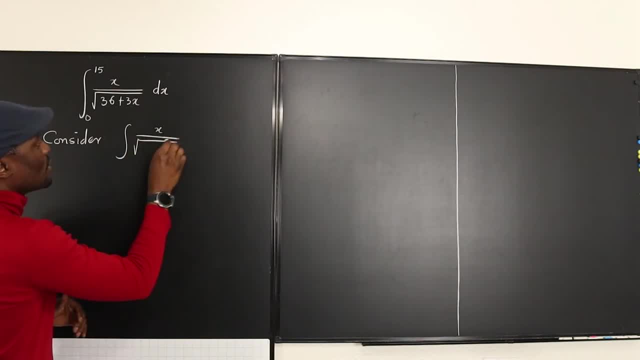 x over b. So we're going to say to consider, because we don't want to keep taking this, 0 and 15 together, square root of 36 plus 3x dx. So this is what we want to deal with. okay, You don't want to keep? 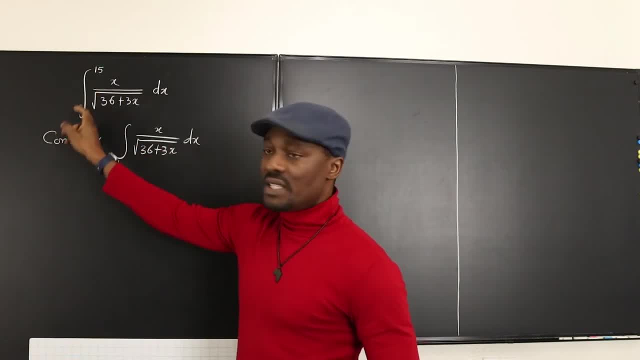 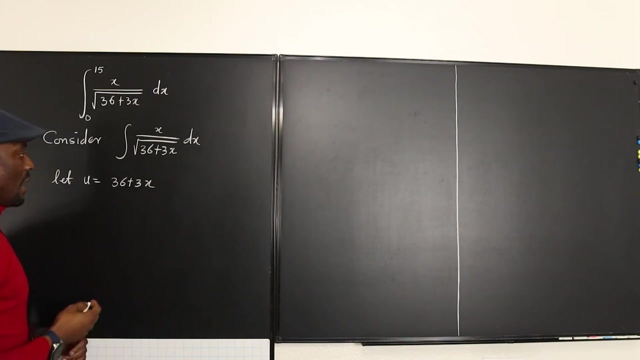 writing this. So, in order to avoid repeating this, just rewrite the expression without that and then, when you're done, you can come back to it. okay, We can say: let u be equal to 36 plus 3x. okay, Whenever you do a? u substitution, it's always good. to have a square root of 36 plus 3x dx. So this is what we want to deal with. okay, You don't want to have a square root of 36 plus 3x dx. So this is what we want to deal with. okay, You don't want to. 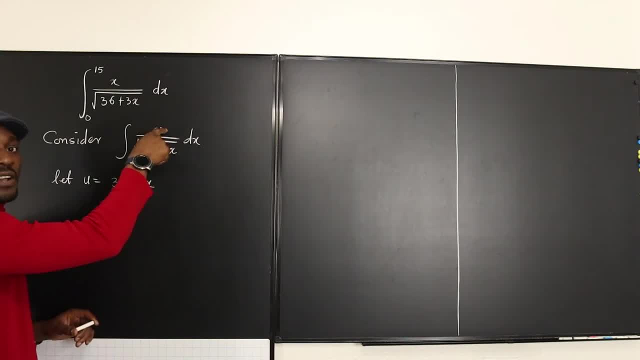 and you find out that this same x you're substituting is somewhere else. You want to know what this x is going to be in terms of u. So that's the first thing you want to do, and that means that x will be u minus 36 divided by 3.. So you want to do that. Okay, that's the first decision you want to make. 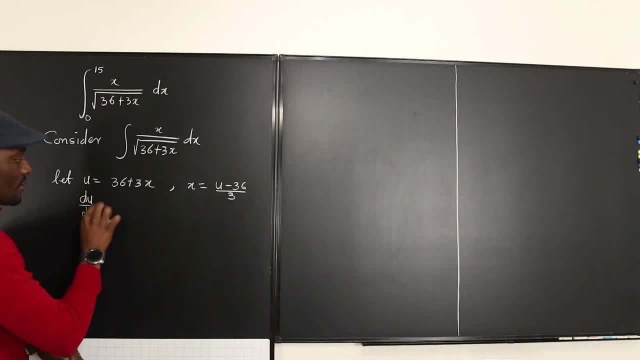 That's done. Now, what's du dx? If we differentiate this, we're going to get 3 and and- because you're going to be writing this, x over b. So you want to do that. So you want to do that. So you want to do. 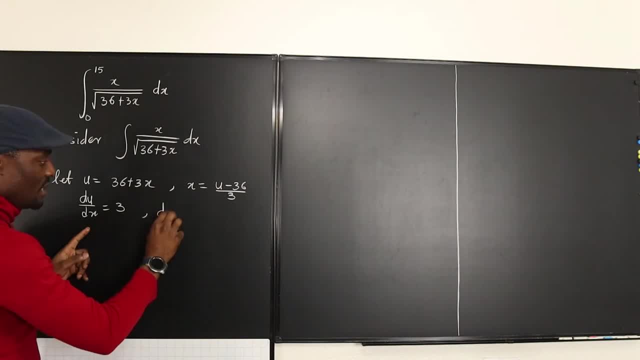 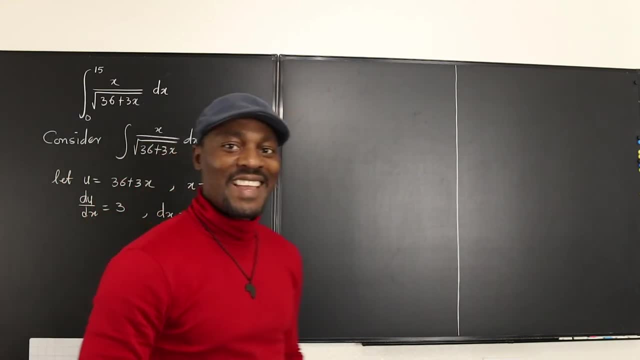 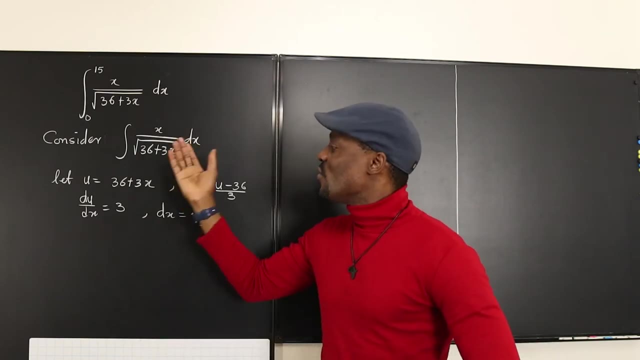 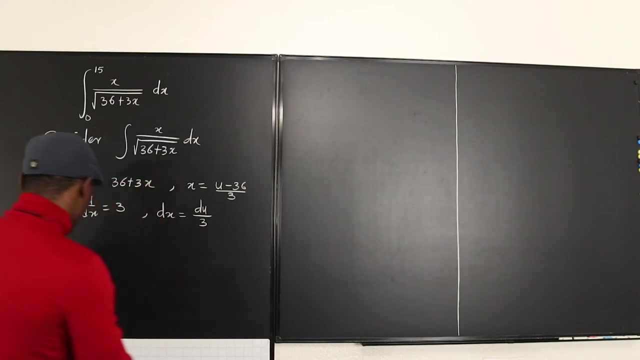 replacing dx for your u substitution. What will dx be? dx will be equal to du over 3.. See, this is what you call the preparation stage. okay, Because if you get this right, you're good. So you can go back and say that this is actually a transformation. So we can say: 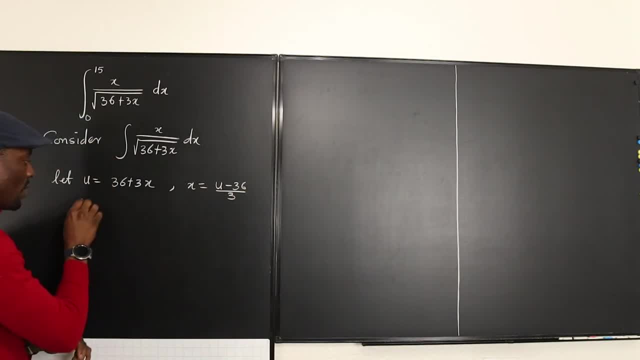 Okay, that's the first decision you want to make. That's done. Now, what's du dx? If we differentiate this, we're going to get 3.. And because you're going to be replacing dx for your u substitution, what will dx be? dx will be equal to du over 3.. 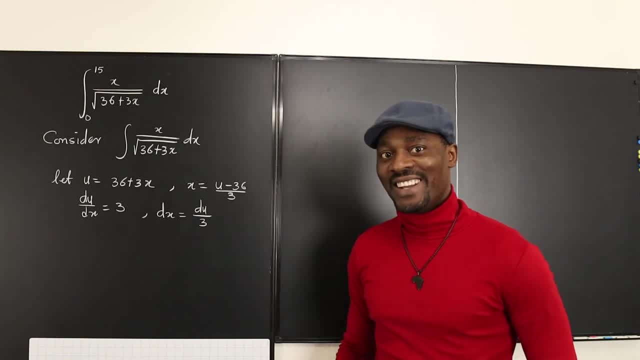 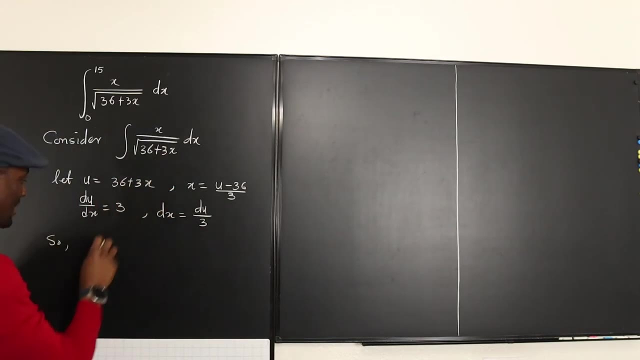 See, this is what you call the preparation stage. okay, Because if you get this right, you're good. So you can go back and say that this is actually a transformation. So we can say that this integral of x over square root of 36 plus 3x dx is actually the integral, or it implies you may not write. 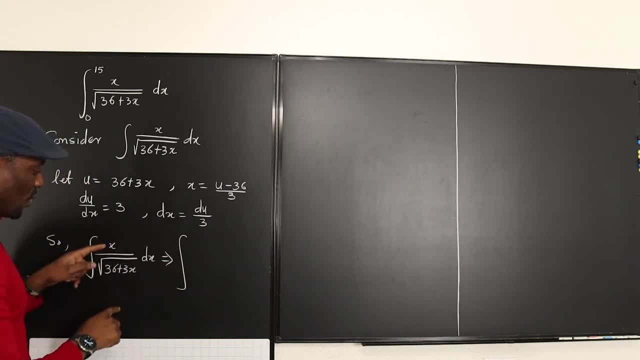 equation. it implies we're going to change all of this. What is x? We said x is this: is u minus 36 over 3 divided by the square root of this? Remember we said this: is u okay? divided by the square root of u. 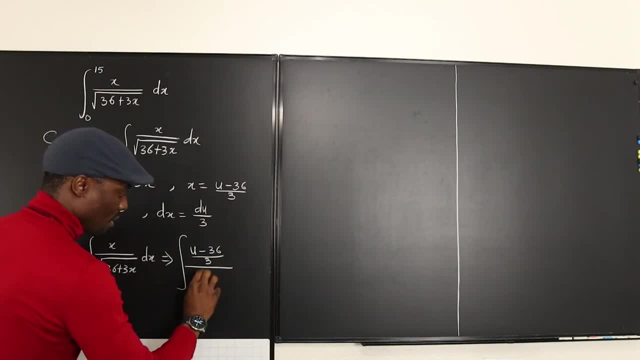 Remember we said this: is u- okay, divided by the square root of u? Okay of u. and what is dx? dx is du over 3, so we just write du over 3. now this is what we need to deal with from now on and we're done with this. okay, now let's go back here. so we're going to go here. 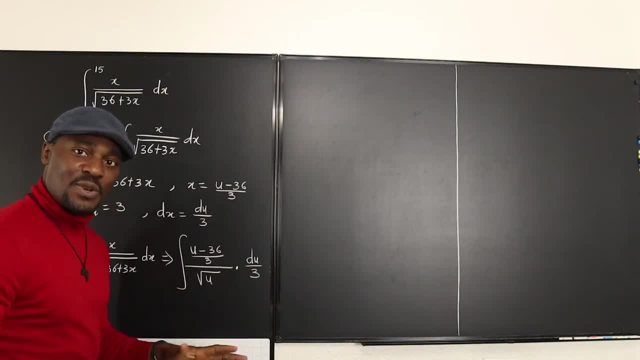 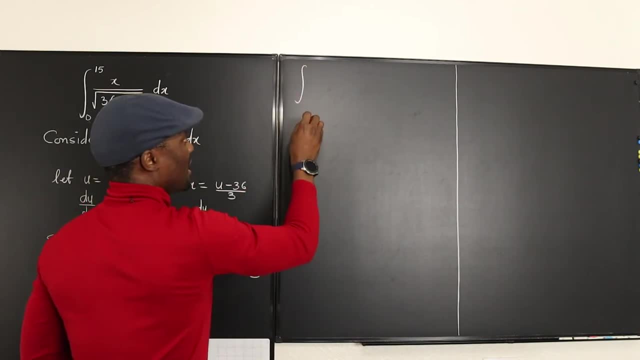 and rearrange this, and this is the rearrangement. this 3 is going to drop down here and this 3 will multiply by 3 and we're going to end up with this integral of u minus 36 over 9 square root of u- du. now this looks cleaner, it's easier, because at this point we can split this into two. this gives: 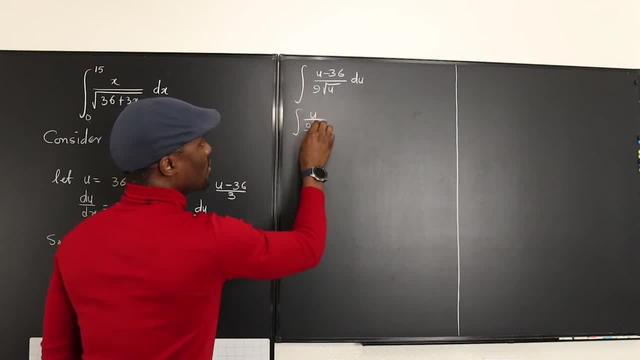 us: u over 9 square root of u, minus 36 over 9 square root of u. okay, du, so we can have two separate integrals from at this point. remember these two are the same, so this can simply mean we have the integral of u over well, u over square root of u. let's clean. 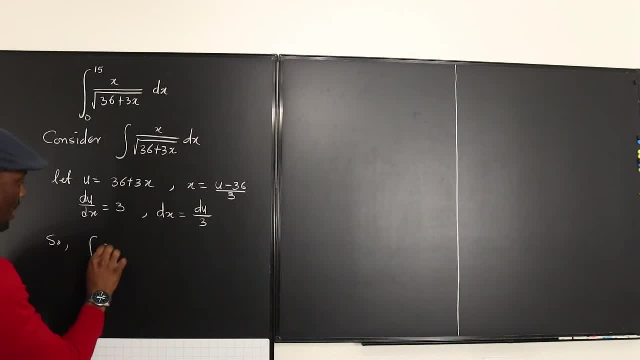 so we can say that this integral of x over square root of 36 plus 3x dx is actually the integral, or it implies you may not write equation is implies we're going to change all of this. What is x? We said x is this: is u minus 36. 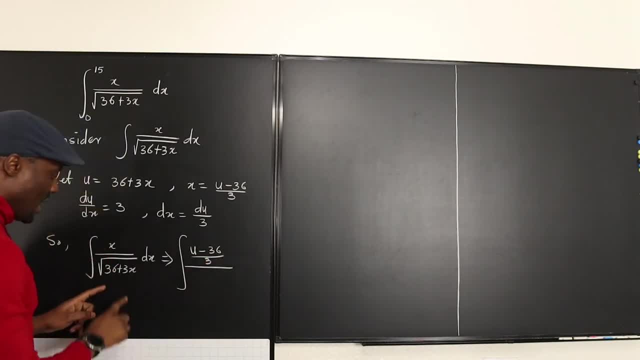 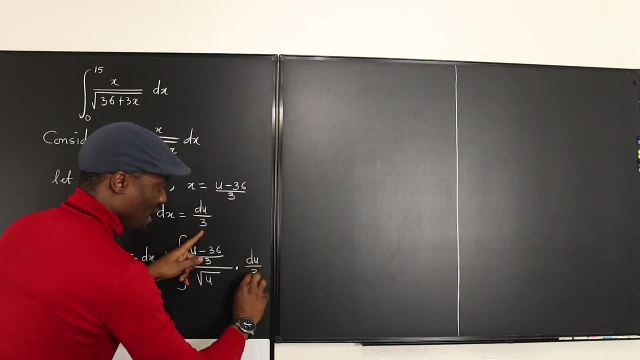 over 3, divided by the square root of this. remember, we said this: is u, okay, divided by the square root of u. and what is dx? dx is du over 3, so we just write du over 3. now, this is what we need to deal with from now on and we're done with this. okay, now let's go back here. so we're going to go here. 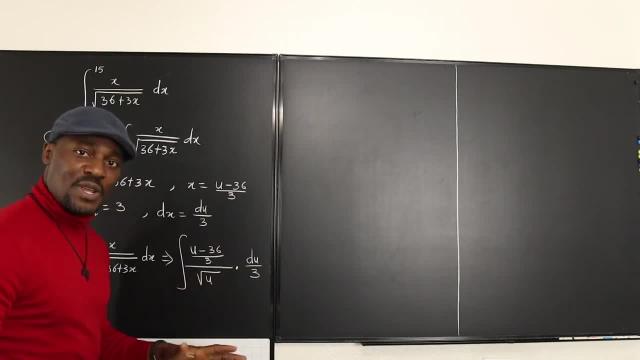 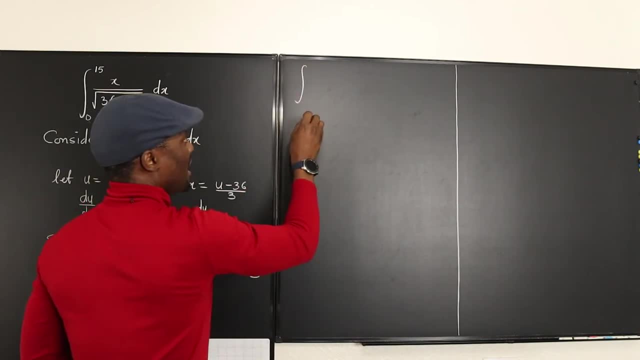 and rearrange this, and this is the rearrangement. this 3 is going to drop down here and this 3 will multiply that 3 and we're going to end up with this integral of u minus 36 over 9 square root of u- du. now this looks cleaner, it's easier, because at this point we can split this into two. this gives: 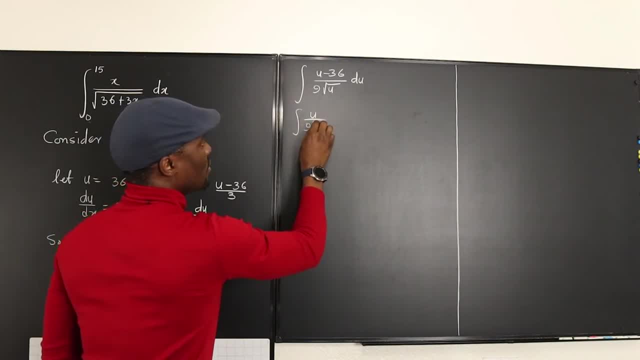 us: u over 9 square root of u, minus 36 over 9 square root of u. okay, du, so we can have two separate integrals from at this point. remember these two are the same. so this can simply mean we have the integral of u over well, u over square root of u. let's clean that up right now. remember that u over. 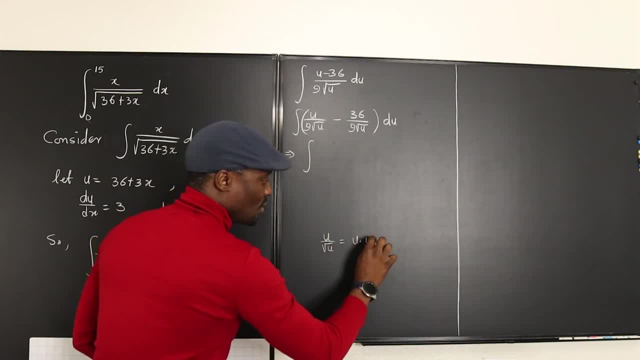 square root of u minus 36 over 9. square root of u minus 36 over 9. square root of u minus 36 over 9. square root of u is the same thing as u times u to the negative one half. okay, if you apply the. 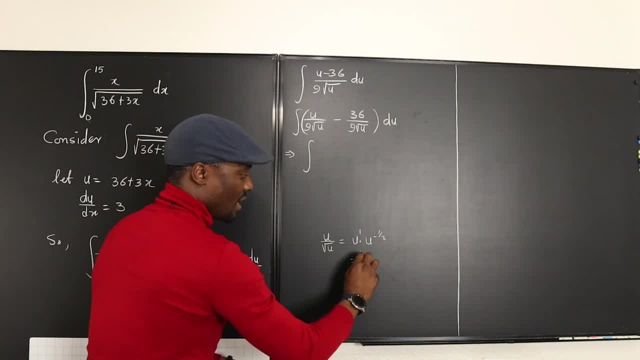 product rule. one minus half is going to give you one half. okay, and that's it. so this is the same thing as 1 over 9 times u to the one half du minus. we do the same thing here too. it's going to be: the integral of 9 in 36 is 4, so it's going to be 4 times u to the negative one half. so we're. 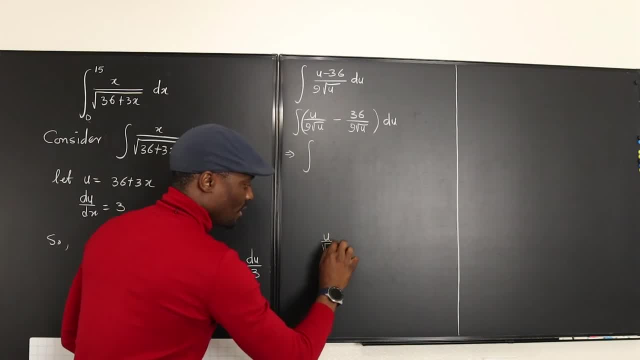 that up right now. remember that u over square root of u is the same thing as u times u to the negative one half. okay, if you apply the product rule, you're going to get u over 9. square root of u minus 36 over 9. square root of u minus 36 over 9. 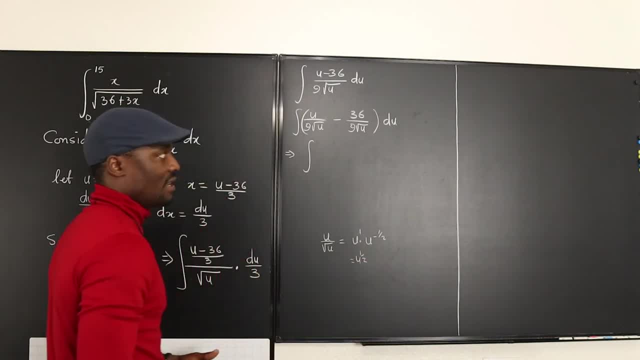 square root of u minus half is going to give you one half, okay, and that's it. so this is the same thing as 1 over 9 times u to the one half du minus. we do the same thing here too. it's going to be the. 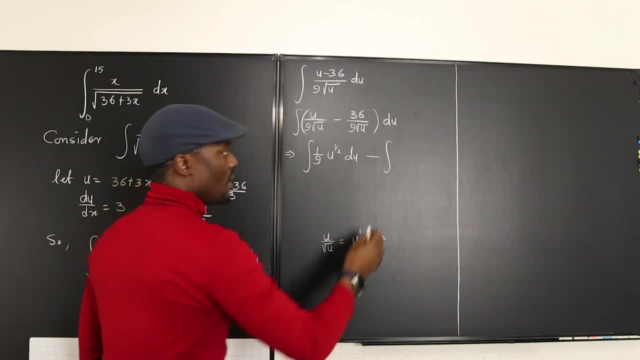 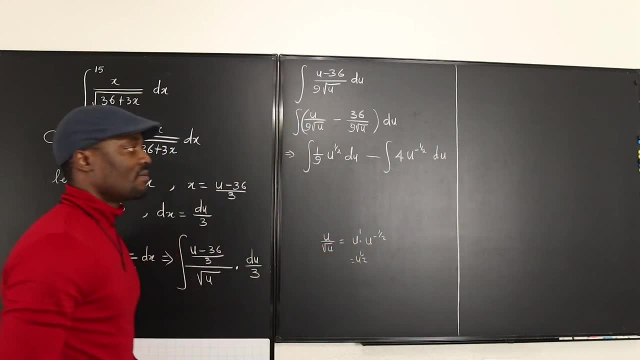 integral of 9 in 36 is 4, so it's going to be 4 times u to the negative one half. okay, du, we just have two expressions now we're writing them in ways that we can easily integrate and that's the most important thing. so, after this separation, 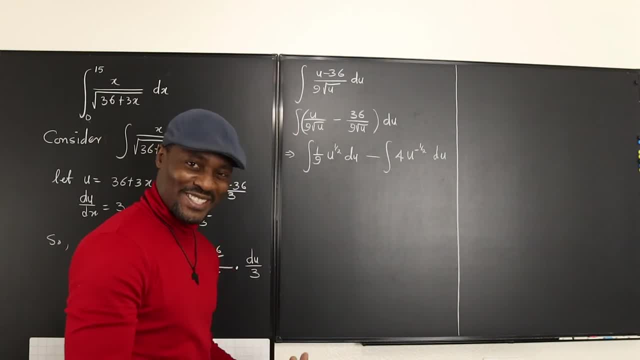 and simplification. the next thing is integration, so let's just integrate, okay? so at this point i'm going to move these constants out, because you don't need them inside. take them outside and they're going to be 1 over 9. the integral of u to the one half du minus 4 multiplied by the. 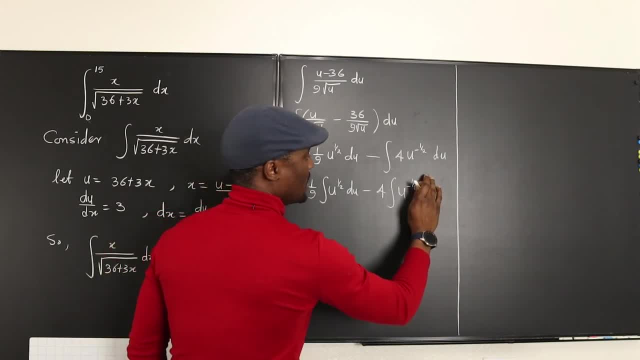 integral of u to the negative 1 over 2 du. and that's it. so let's just integrate. okay, so at this point i'm going to move these constants out, du. oh, this goes here. okay, let's integrate. if you integrate this, you're going to add one to it. 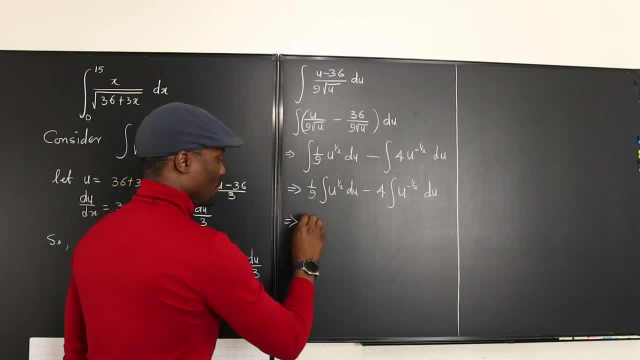 that's going to be 3 over 2, and then you divide by 3 over 2, so this is going to be 1 over 9. okay, times u watch this, i'm going to leave a space here. times u to the 3 over 2. 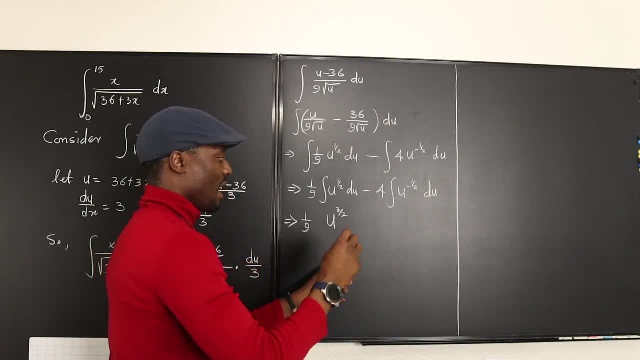 divided by 3 over 2, but that means multiplied by 2 over 3, times 2 over 3. that's a quick trick. minus you do the same thing here. it's going to be 4. leave a space u to the if you add one to. 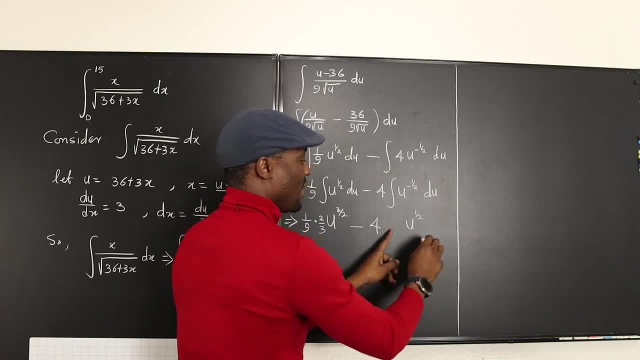 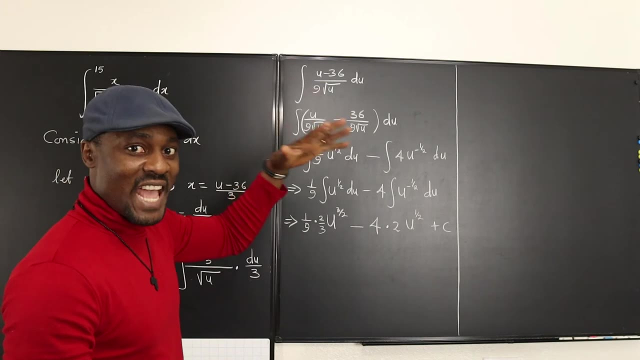 this is going to be one half, that's u to the one. half divided by one half will be the same thing as multiplying by 2. okay, we've done our integration. and plus c. remember, you need to put the plus c at this point because you're not using your boundaries yet. okay, so when your boundaries are not in effect, 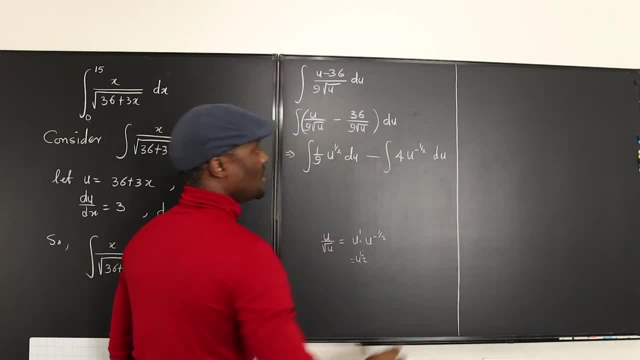 going to have a negative one half. okay, du. we just have two expressions now. we're writing them in ways that we can easily integrate, and that's the most important thing. so, after this separation and simplification, the next thing is integration. so let's just integrate, okay. so at this point i'm 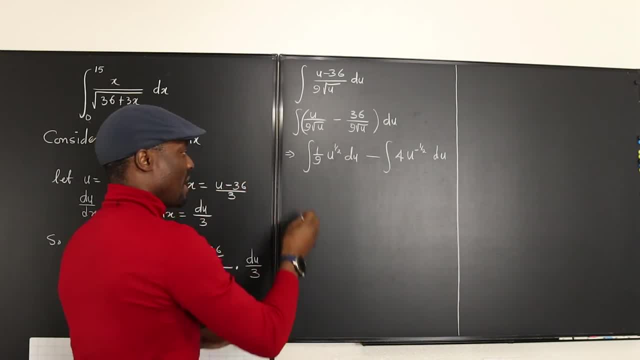 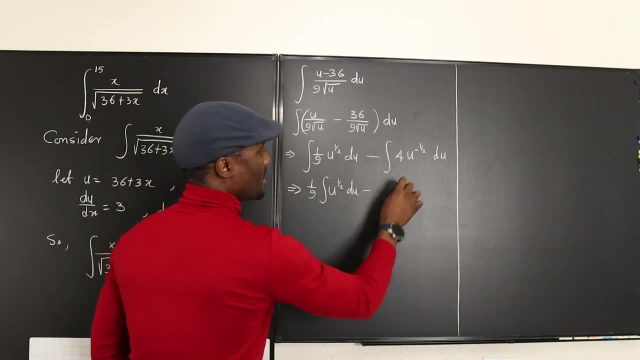 going to move these constants out because you don't need them inside. take them outside and they're going to be 1 over 9. the integral of u to the one half du minus 4, multiplied by the integral of u to the negative, 1 over 2 du. oh, this goes here. 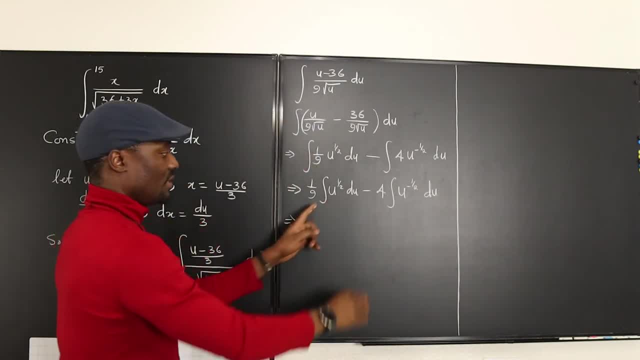 okay, let's integrate. if you integrate this, you're going to add 1 to it. that's going to be 3 over 2, and then you divide by 3 over 2, so this is going to be 1 over 9. okay, times u watch this, i'm going. 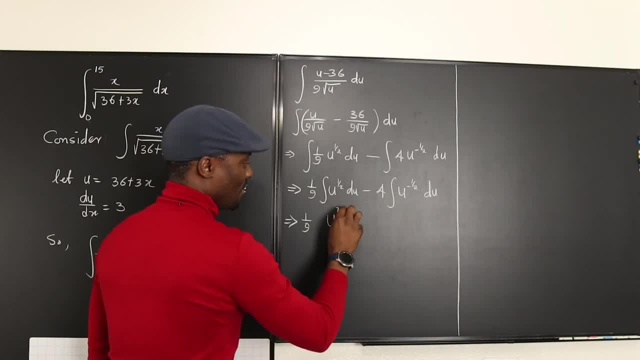 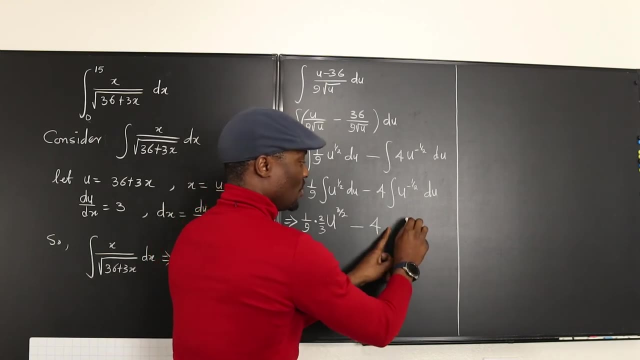 to leave a space here. times u to the 3 over 2, divided by 3 over 2. but that means multiplied by 2 over 3, times 2 over 3. that's a quick trick. minus you do the same thing here, it's going to be 4. leave a space u to the. if you add 1 to this is: 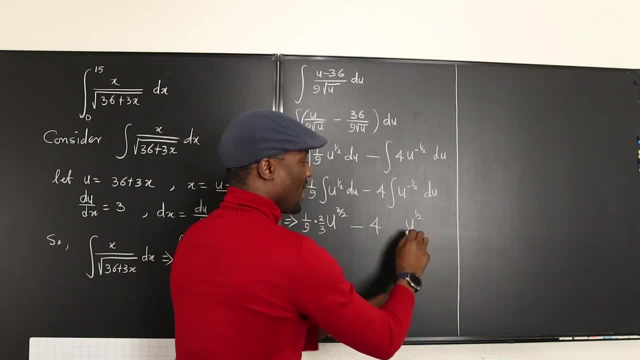 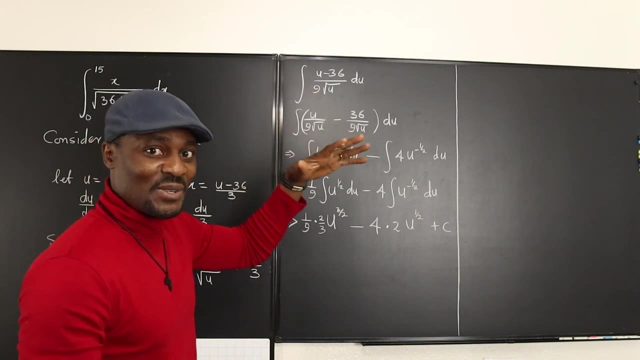 going to be 1 half, that's u to the 1 half. divided by 1 half will be the same thing as multiplying by 2. okay, we've done our integration. and plus c. remember, you need to put the plus c at this point. you don't need to put the plus c because you're not using your boundaries yet, okay, so when your 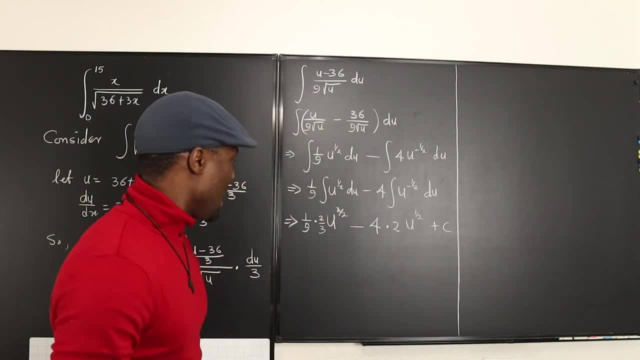 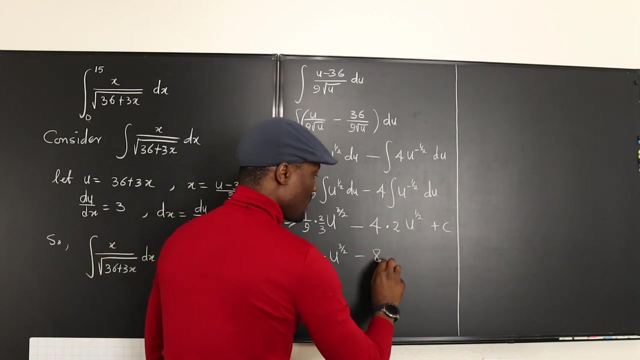 boundaries are not in effect. you have to remember to put the plus c um. let's clean this up and see what our substitutions will be. so this will be the same thing as u to the over 27, so this is going to be 2 over 27. u to the 3 over 2 minus. at this point it's going to be 8: u to the one half. okay, that's. 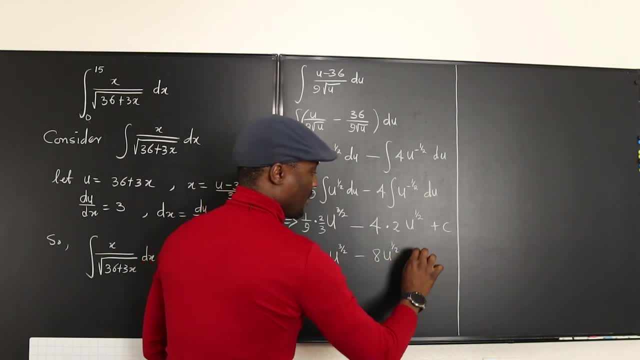 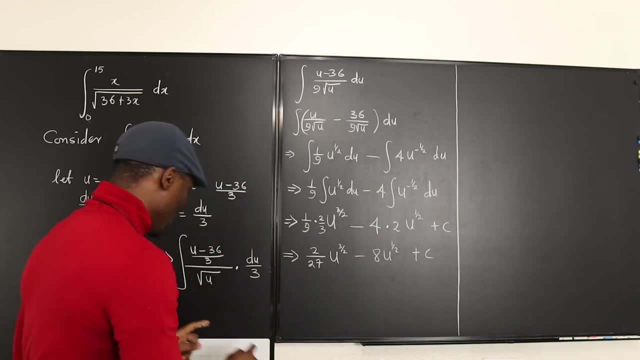 the square root, but let's just make it 1 half, okay, plus C. now that we're done integrating, we've gotten you. let's go back to this equate. no, this equation we started with and put the boundaries, now your boundaries. this is where many people forget. your boundaries will no longer be in terms of X, like we started. 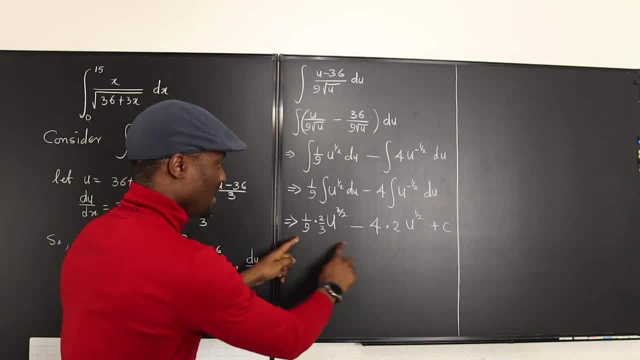 you have to remember to put the plus c. let's clean this up and see what our substitutions will be. so this will be the same thing as u to the over 27. so this is going to be 2 over 27. u to the 3 over 2 minus. at this point it's: 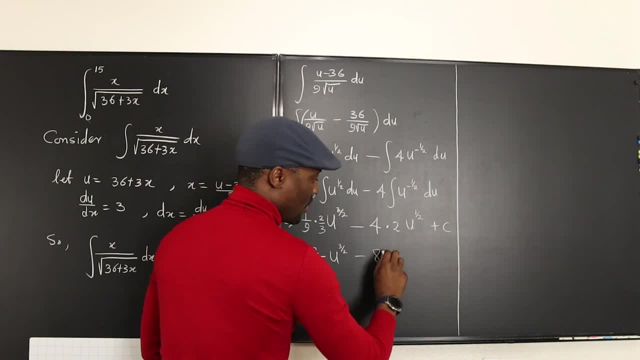 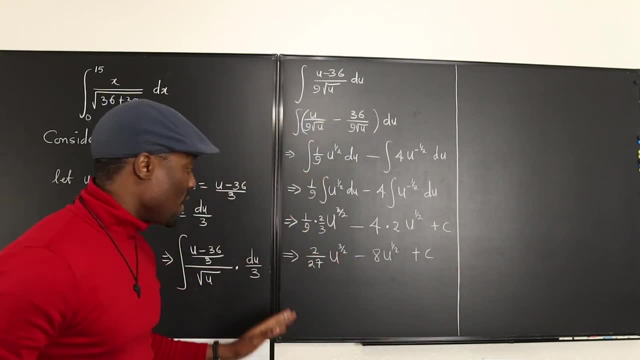 going to be 8: u to the one half. okay, that's the square root, but let's just make it one half, okay, plus c. now that we're done integrating, we've gotten u. let's go back to this equation. no, this equation we started with and put the boundaries, now your boundaries. this is where many people forget your boundaries will. 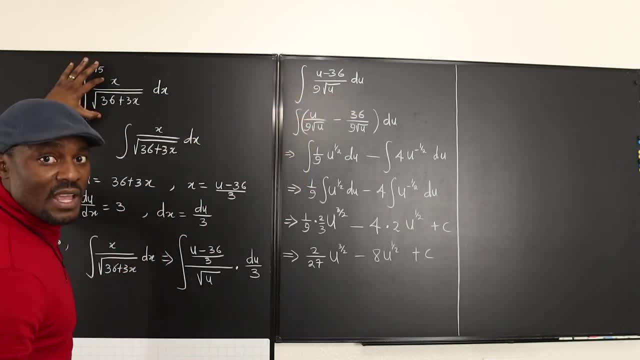 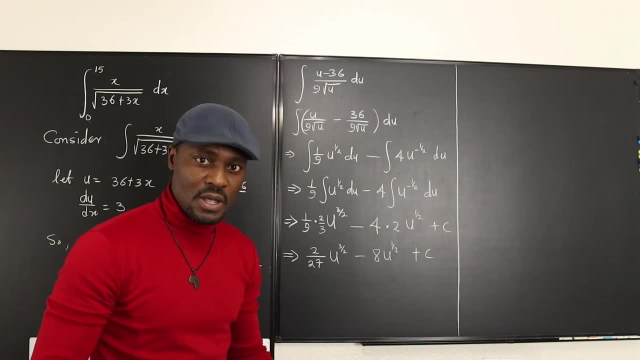 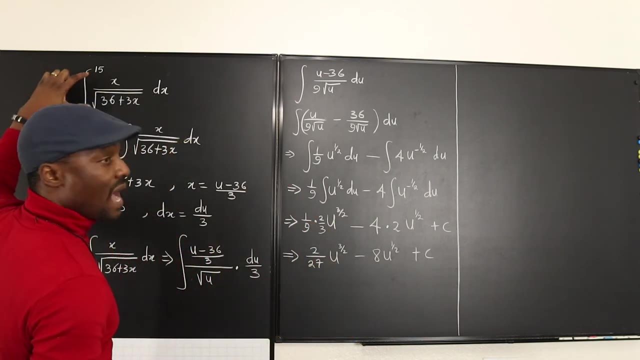 no longer be in terms of x, like we started with the boundaries, are going to be in terms of u, because you have integrated with respect to u. so what is u when x is 0 and what is u when x is negative? u times u or pi, Kха, e, J. 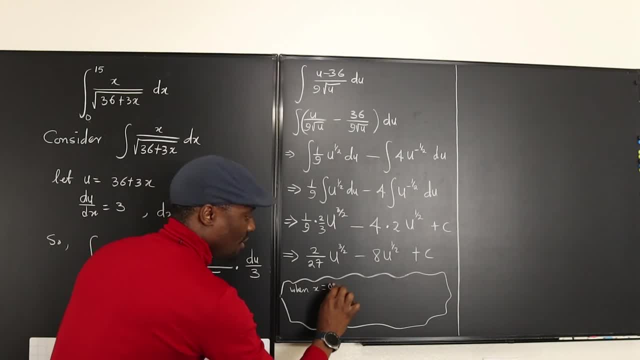 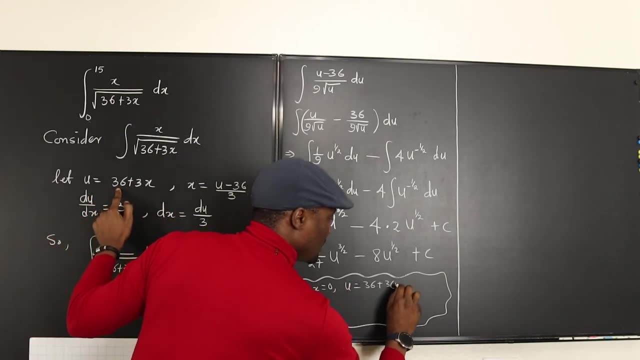 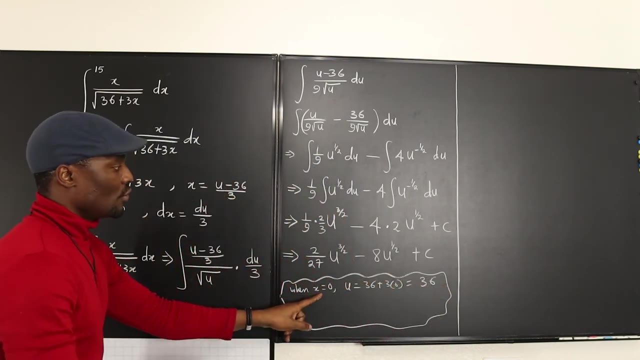 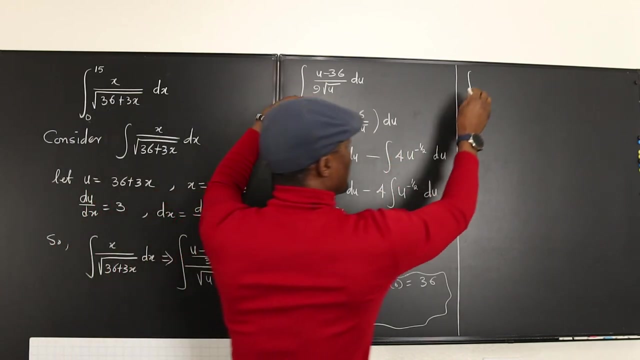 all right times u goes to x. so if you tried that first time, you have a probability that x will be 0, because u matches old 1, 2, 3, 4, 5, 6, this expression here, which is um, you know what i'm going to take this 9 to the other side. no, 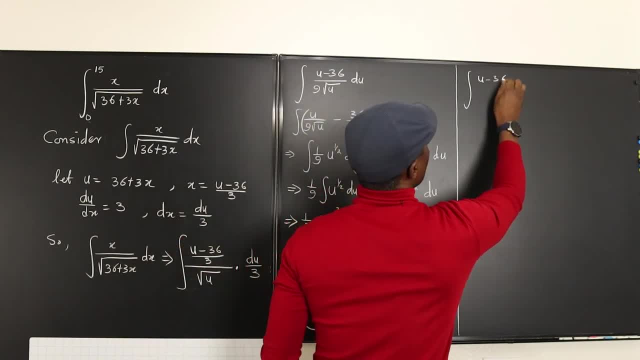 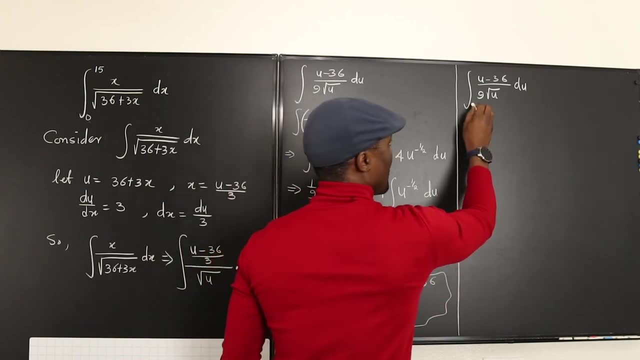 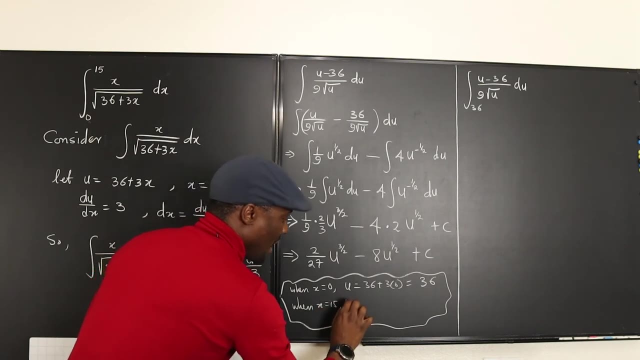 just leave it inside: u minus 36 over 9, square root of u, du, with a lower boundary of 36 and an upper boundary. let's find the upper boundary. when x equals 15, you have u equals 36 plus 3 into 15, that's 45 plus 36. that's going to give you 81. the upper boundary is 81. now, never. 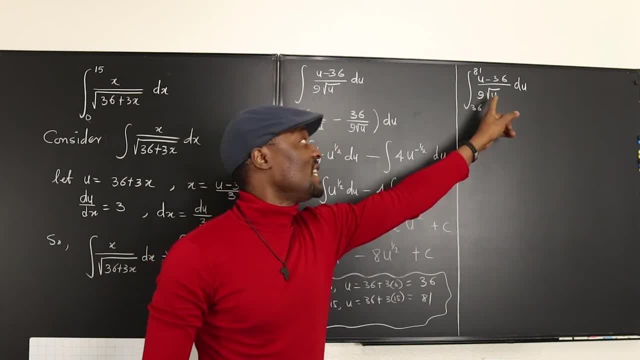 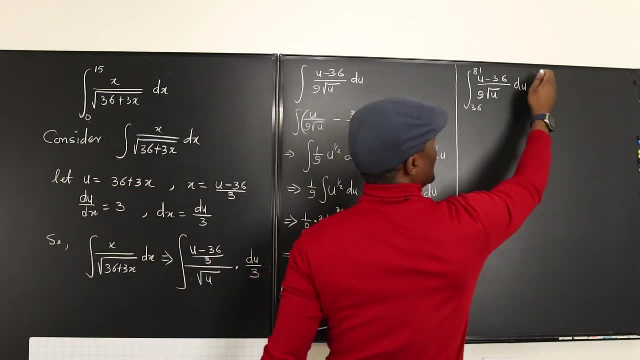 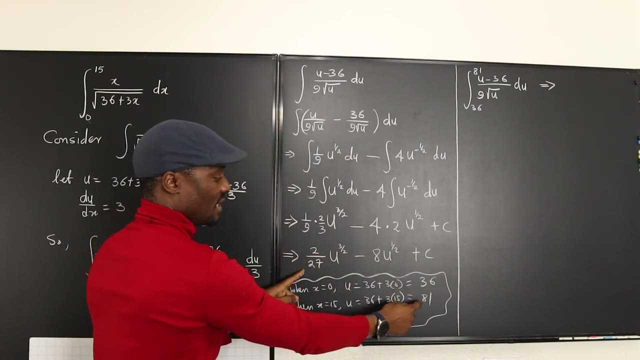 forget to do this, because if you plug in 0 and 15 into this, into this value for your evaluation, that's going to be a problem. okay, so this expression actually gives us this, and then we evaluate at these limits: 36 and 81. okay, so this will now. 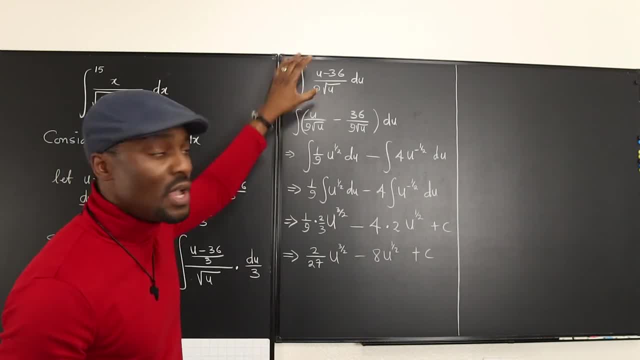 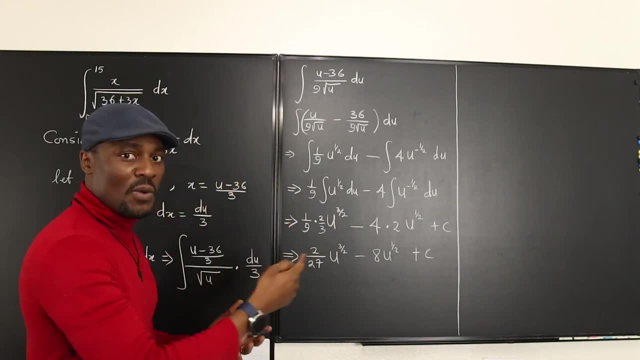 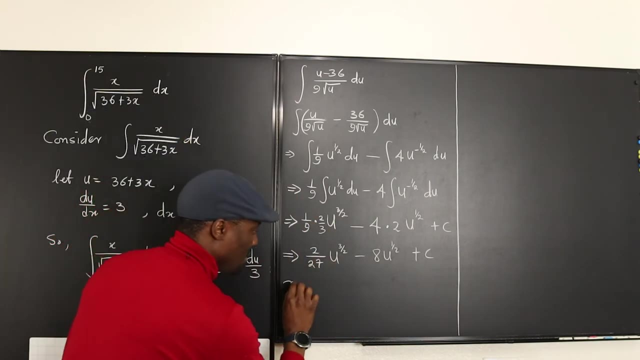 with the boundaries are going to be in terms of you, because you have integrated with respect to you. so what is U when X is 0 and what is U when X is 15? those are the two boundaries. so you quickly do your math here. just create a box. I'm going to create a box here. okay, so when X equals 0, you. 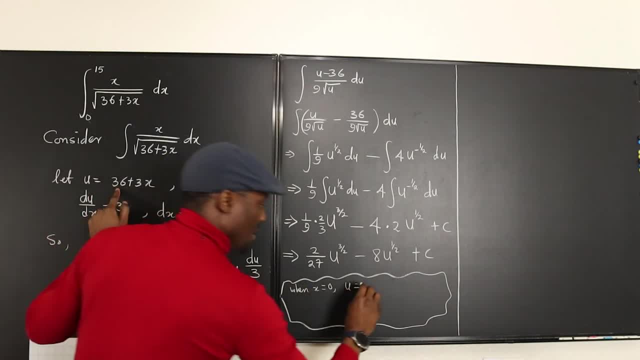 will be equal to 36 plus 36 plus 3 into 0, and that would give us 36 plus 0. that gives us a balance X, 0, y. assuming you create a box, word box- here and you have gives us 36.. So that's our lower boundary, remember? So that's what we're going to write. 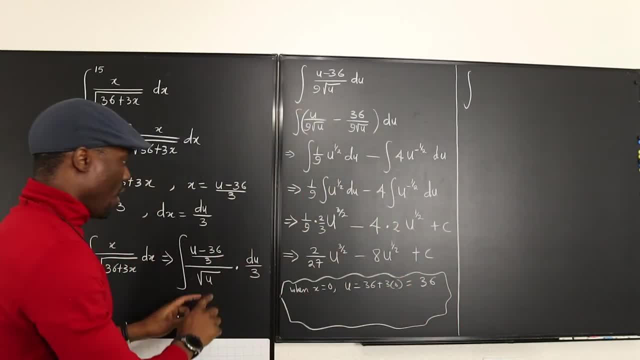 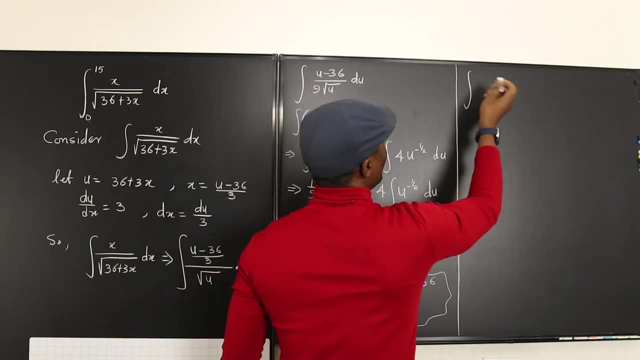 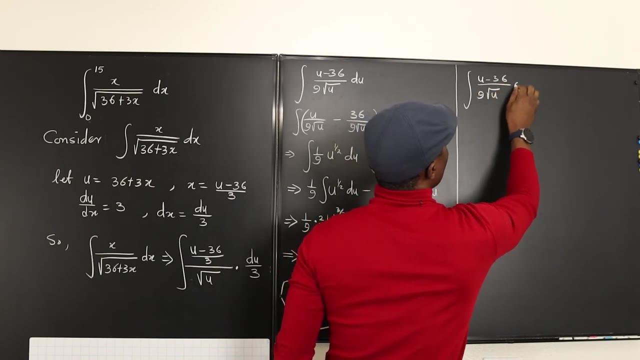 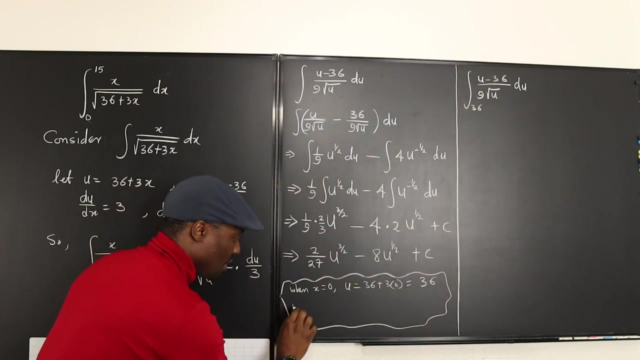 here and say that the integral of this expression here, which is you know what I'm going to take this 9 to the other side. No, just leave it inside: u minus 36 over 9 square root of u du, with a lower boundary of 36 and an upper boundary. Let's find the upper boundary. 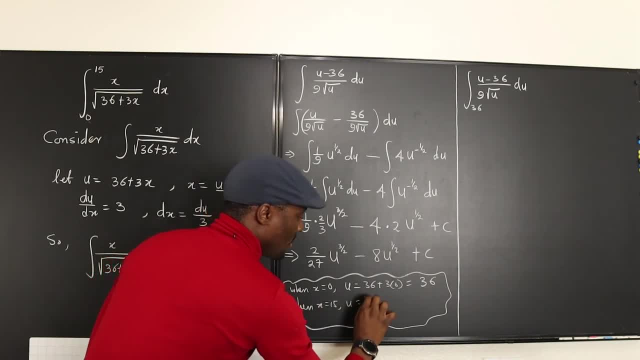 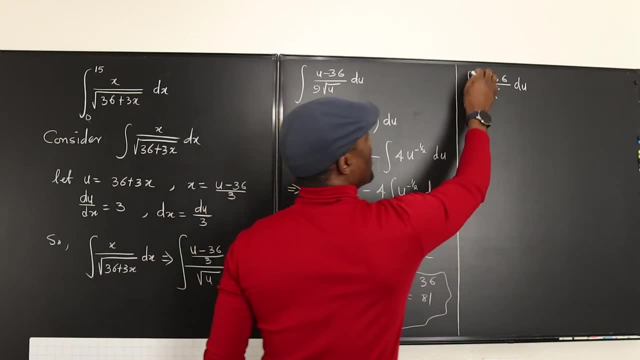 When x equals 15, you have: u equals 36 plus 3 into 15.. That's 45 plus 36.. That's going to give you 81.. The upper boundary is 81.. Now, never forget to do this, because if you plug in 0 and 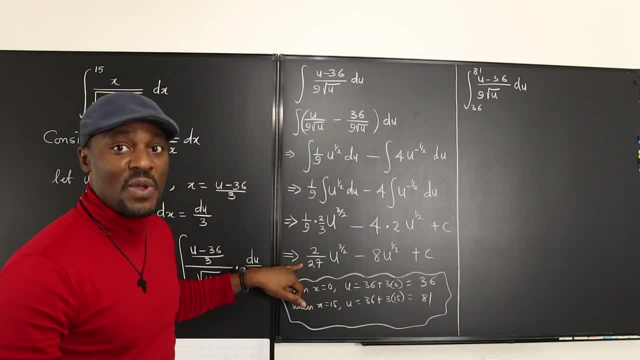 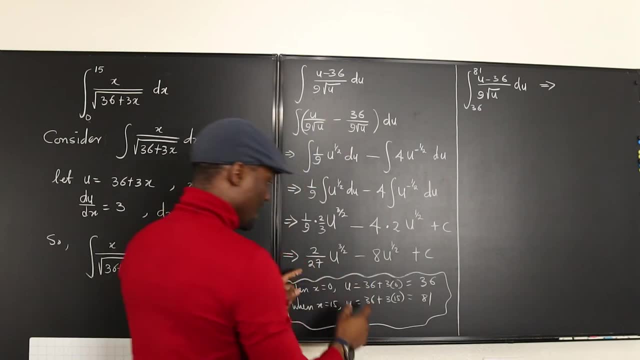 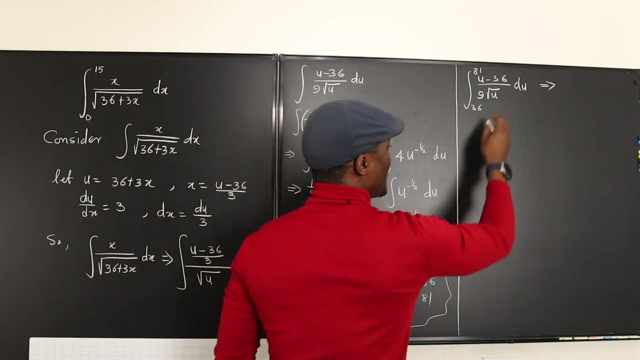 15 into this, into this value for your evaluation. that's going to be a problem, Okay. Okay, So this expression actually gives us this, and then we evaluate at these limits: 36 and 81.. Okay, So this will now be equal to. you know, we have integrated this, So this is. 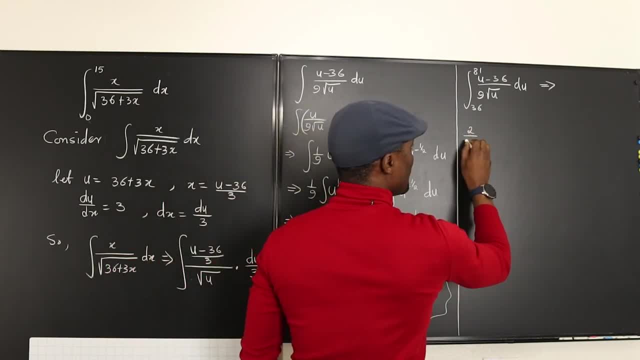 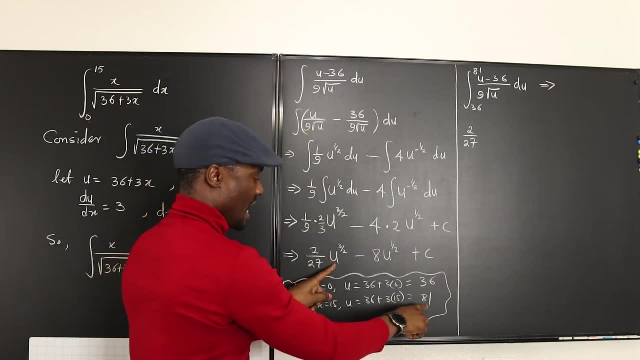 our answer: It's going to be 2 over 27.. Then what is u? u is now? that's: we're going to start with the upper boundary. That's going to be 81.. That's 81 raised to the power of 3 over 2. 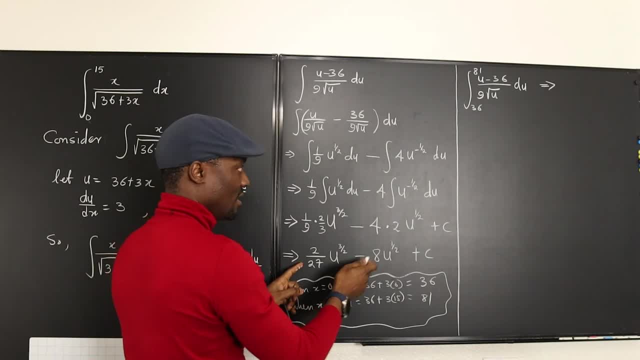 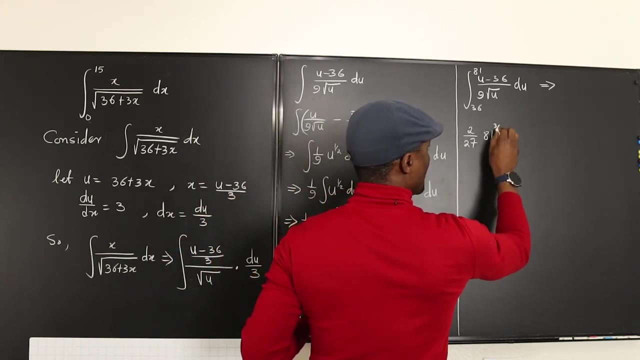 be equal to. you know, we have integrated this, so this is our answer. it's going to be 2 over 27. then what is u? u is now? that's: we're going to start with the upper boundary. that's going to be 81. that's 81 raised to power, 3 over 2 minus. okay, we're multiplying minus 8? u to the half, that's. 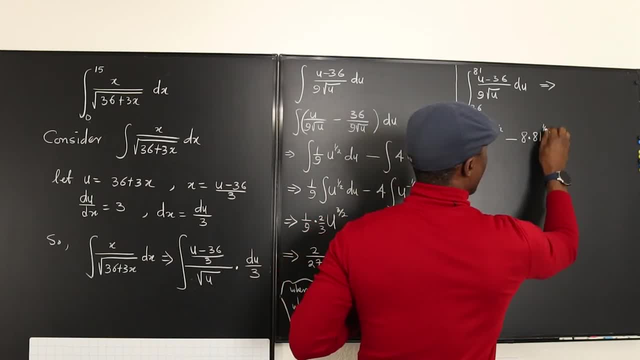 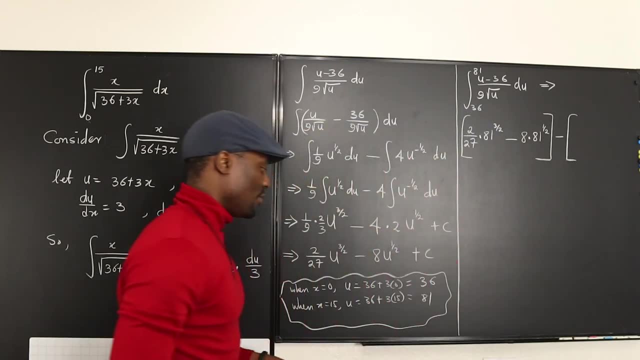 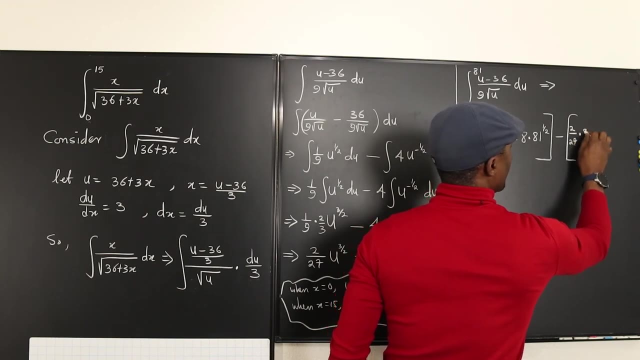 going to be 8 times 81 to the one half. okay, that's the first portion, minus the lower boundary. the lower boundary is using 36. we repeat the same numbers: 2 over 27 times 36, raised to power: 3 over 2 minus 8 times 36 to the one half. okay, so that's. 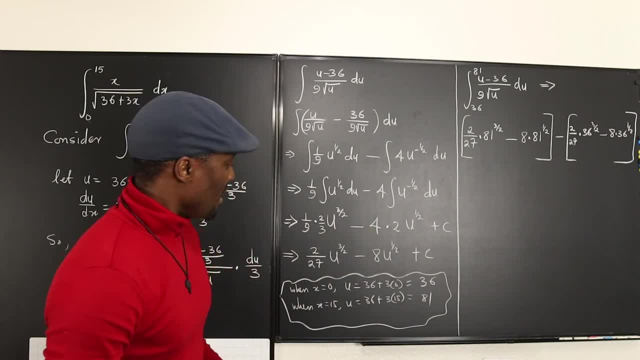 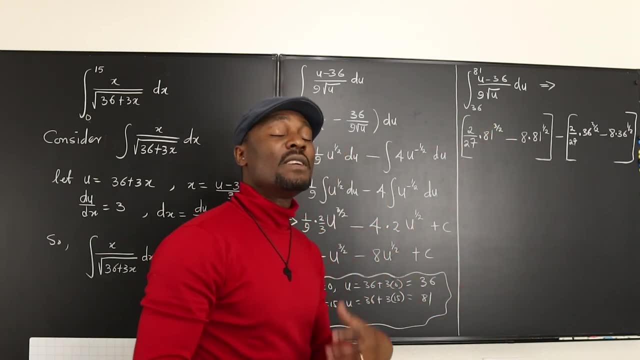 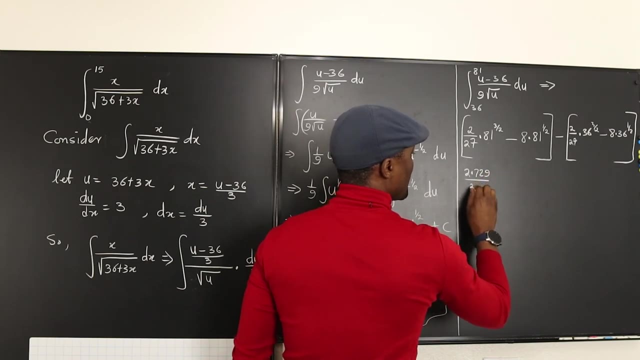 it. let's evaluate. so at this point we're just: the square root of 81 is 9. 9 raised to the third power is 729. so you want to do that. so this is going to be 2 times 729 over 27 minus. this is going to be square root of. 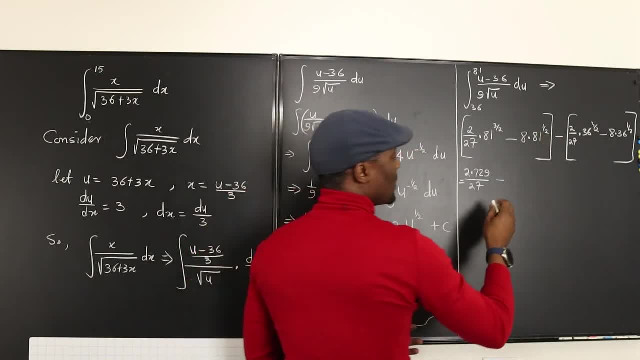 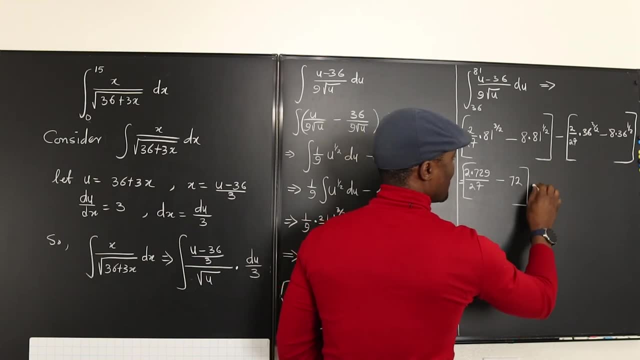 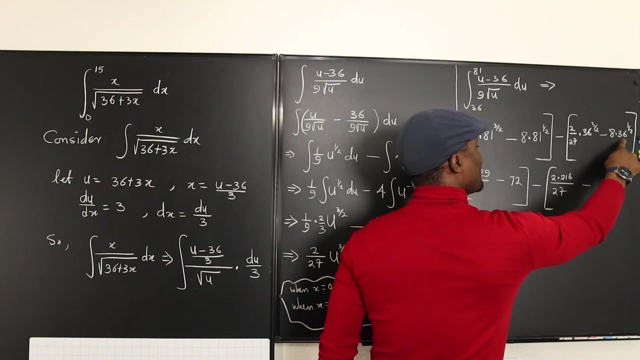 um 81 is 9. 9 times 8 is 72. okay, so we'll put this still in parentheses. okay, just like this Minus, we do the other side- This is square root of 36- is 6.. 6 to the 3rd power is 216.. So that's 2 times 2, 1, 6 over 27.. And this will be minus. this is square root of 36 is 6.. 6 times 8 is 48.. 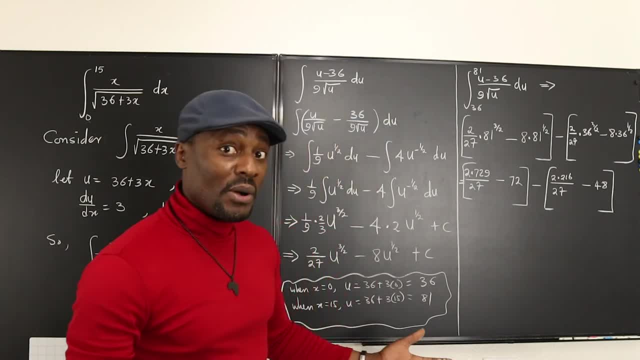 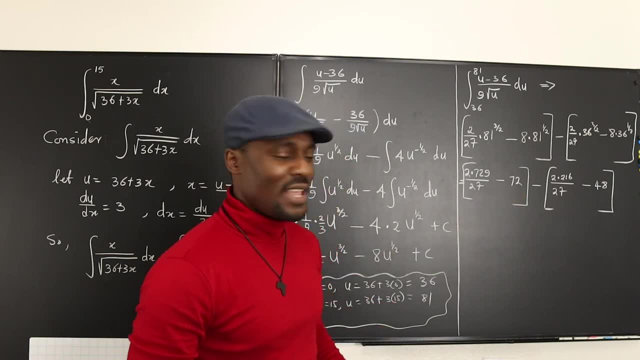 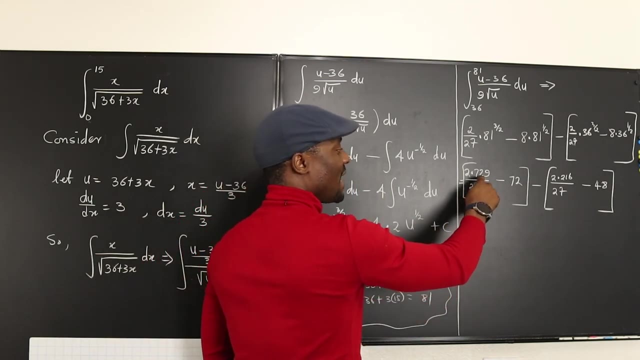 Now some people will start simplifying. You know what? Let's just try and see how well we can simplify this. Let's see: 9 will divide 27, three times 9 will divide this: how many? 81 times. 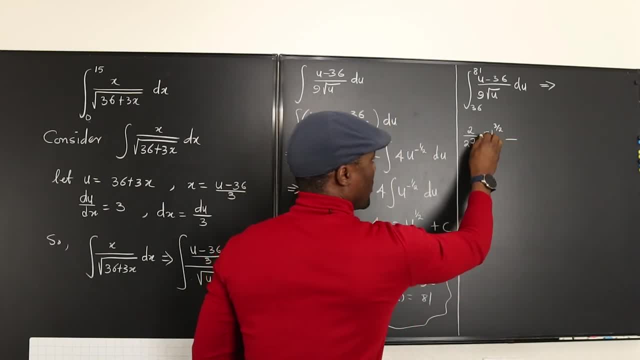 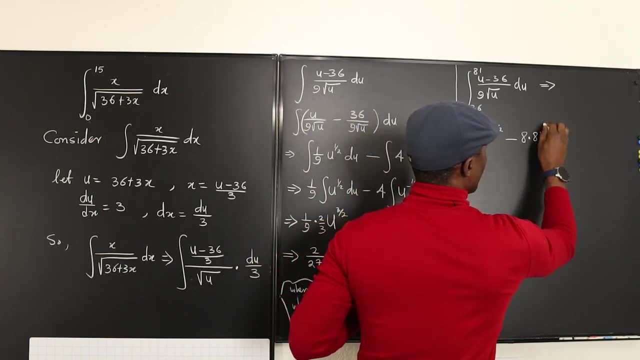 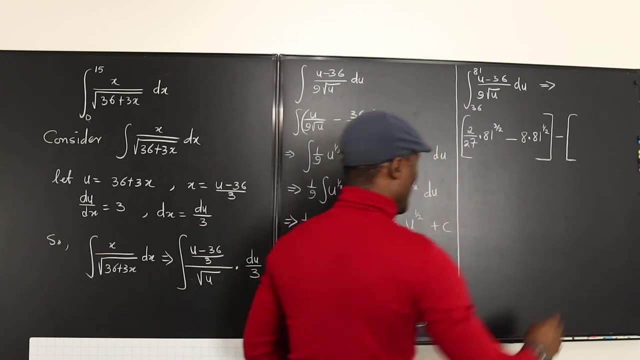 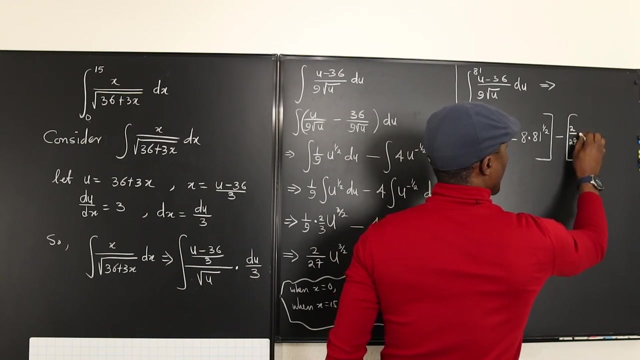 minus. okay, we're multiplying minus 8u to the half. That's going to be 8 times 81 to the one half. Okay, That's the first portion minus the lower boundary. The lower boundary is using 36.. We'll repeat the same numbers: 2 over 27 times 36, raised to the power of 3 over 2. 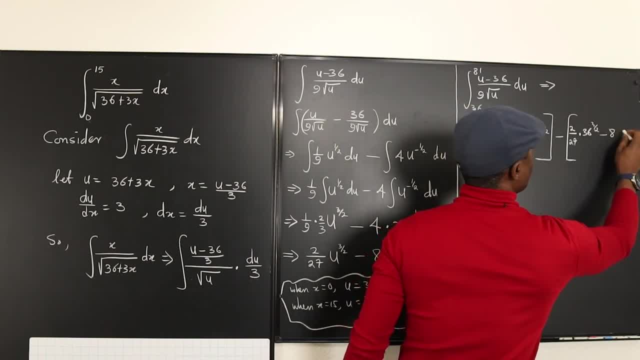 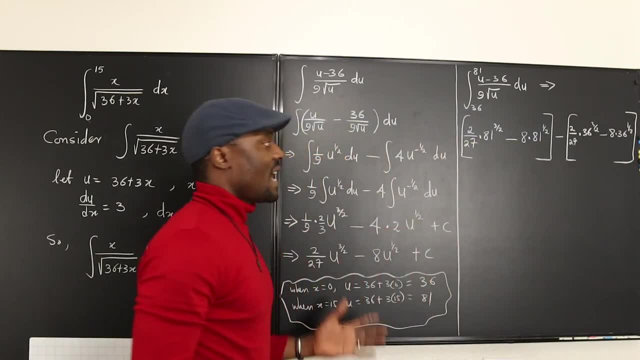 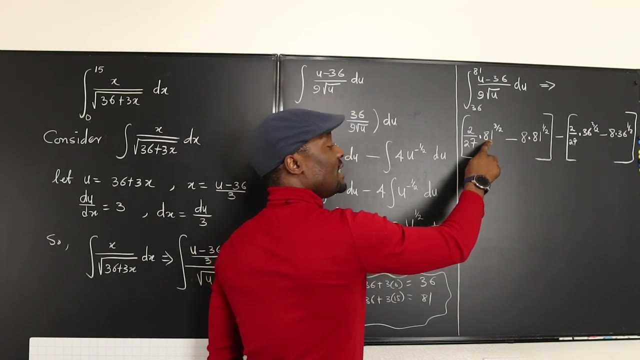 minus 8 times 36 to the one half. Okay, So that's it. Let's evaluate. So at this point we're just: the square root of 81 is 9.. 9 raised to the third power is 729.. So you want to do that? 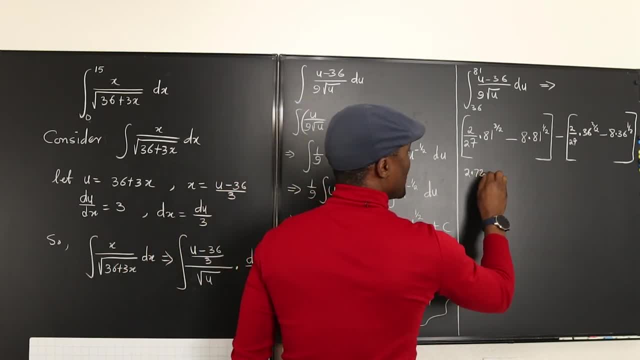 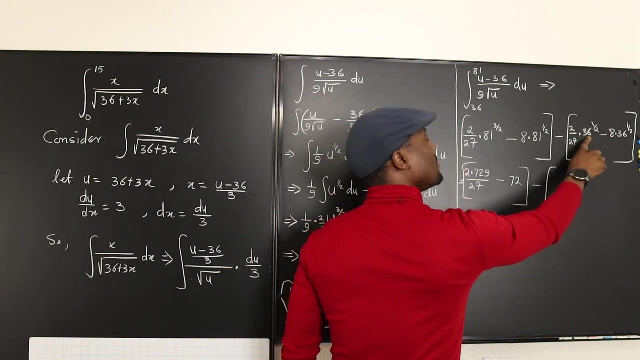 So this is going to be 2 times 729 over 27.. Minus- This is going to be square root of 81 is 9.. 9 times 8 is 72.. Okay, So we'll put this still in parentheses. Okay, Just like this Minus, We do the other side. This is, square root of 36 is 6.. 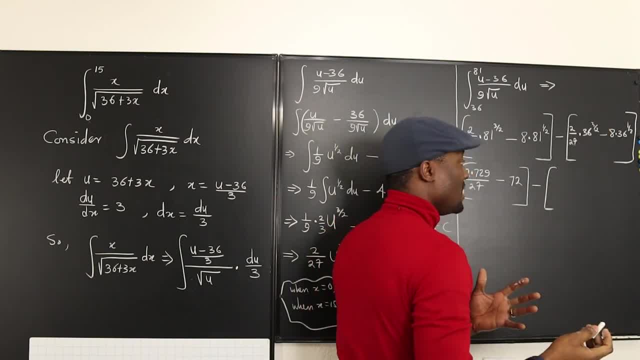 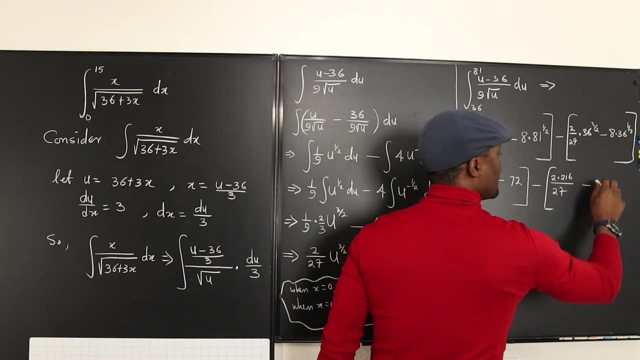 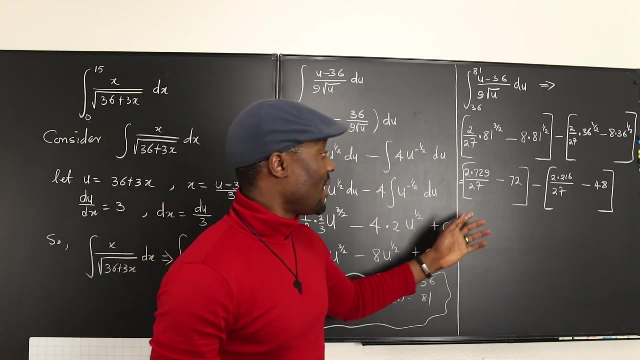 6 times 6 to the third, power is 216.. So that's 2 times 2, 1, 6 over 27.. And this will be minus. This is square root of 36 is 6.. 6 times 8 is 48.. Now some people will start simplifying. 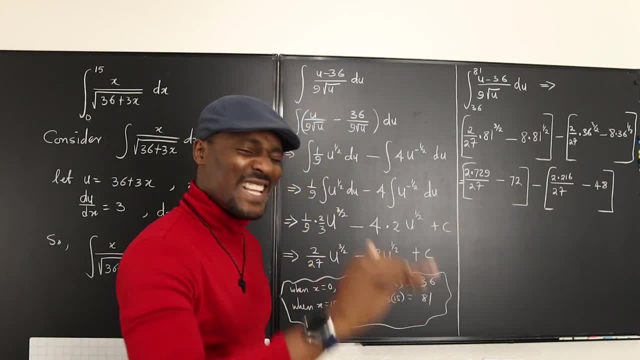 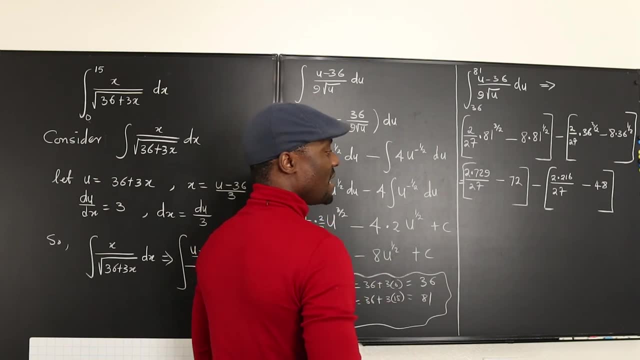 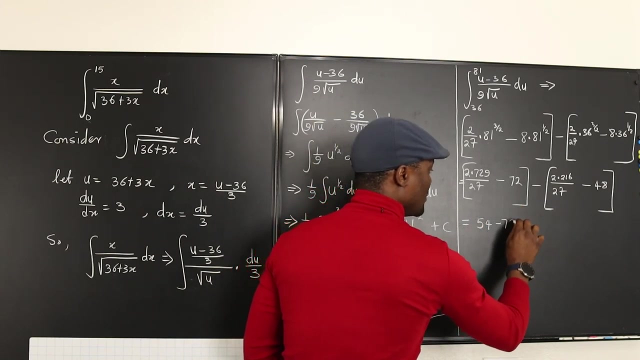 You know what? Let's just try and see how well we can simplify this. Let's see: 9 will divide 27. three times 9 will divide this how many? 81 times? So? 3 in 81 is supposed to be 27.. So 27 times 2 is 54.. Oh, we got that. So this is 54 minus 72 minus. 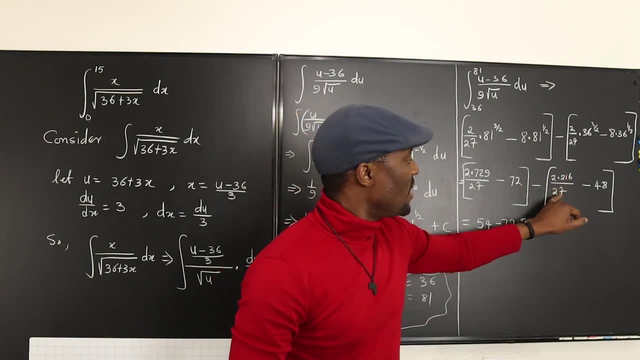 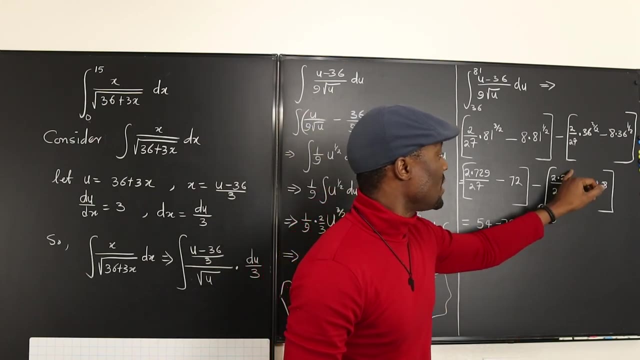 let's see what this gives us. Firstly, I know 3 will divide these two numbers. Okay, So let's start with that. 3 here will give us 9.. And 3 in 216 is going to be 72.. No, 3 in 216 is going to be 72..